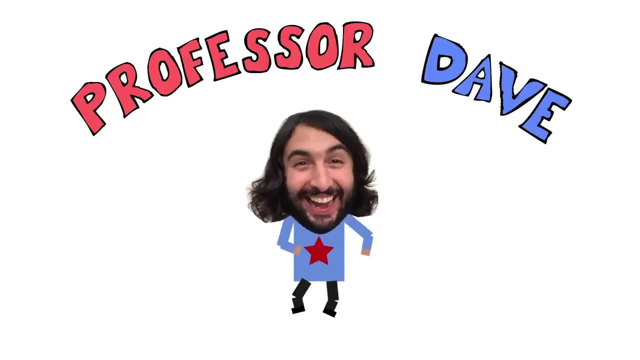 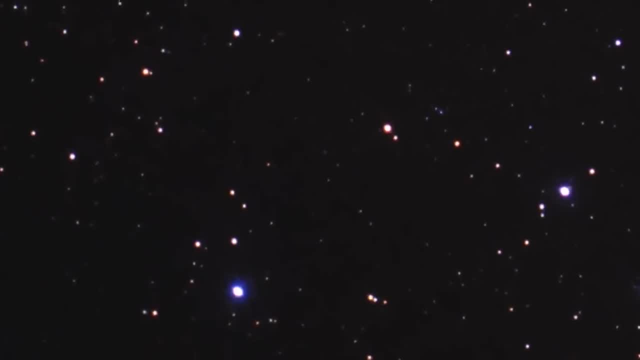 One of the most incredible things about studying the universe is that when we use powerful telescopes to look out into space, we are also looking back in time. The distances between celestial objects are so incredibly vast that the light they emit, even though it travels at the 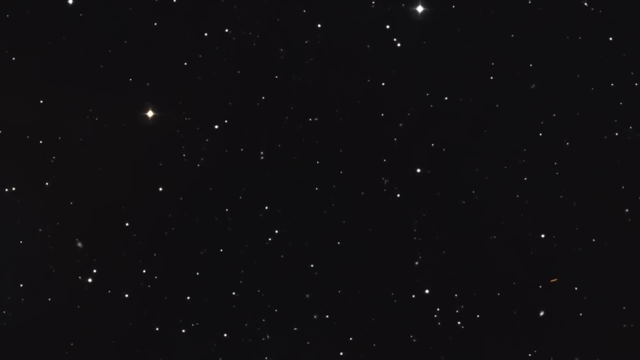 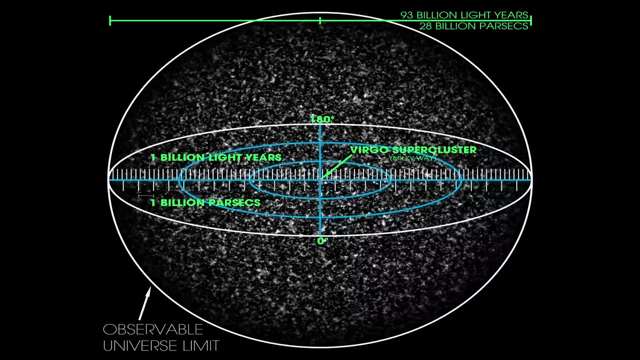 speed of light, which is the fastest speed possible, it still takes many years to get to us And, in the case of objects outside the Milky Way galaxy, it takes millions or even billions of years to get to us. This puts a fundamental limit on how far we can see because, given that the 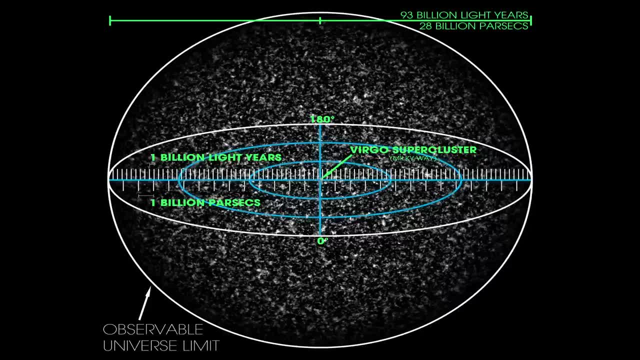 universe began approximately 13.8 billion years ago and then factoring in for the expansion of the universe over its lifetime, it is impossible for us to see farther than approximately 46.5 billion light years away, as light can't have been traveling. 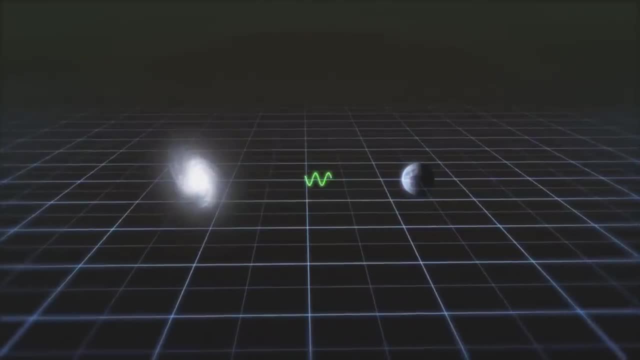 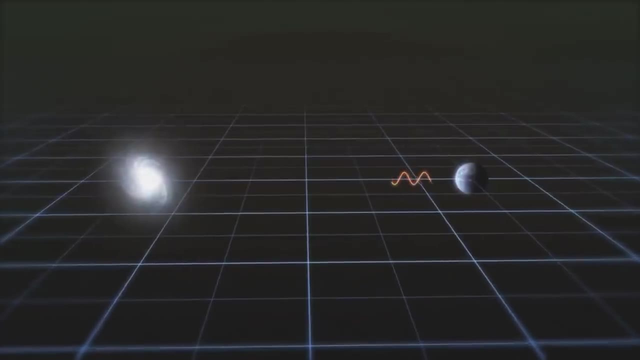 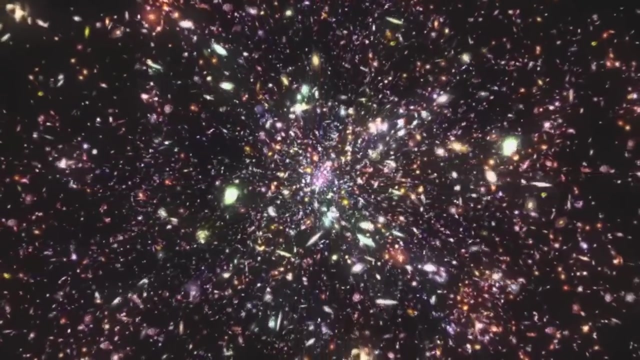 for longer than the universe has existed. a limitation that does not change, even though the universe has expanded significantly during that time, which changes the wavelength of that light in predictable ways. The finite length of time into the past for the birth of the universe. 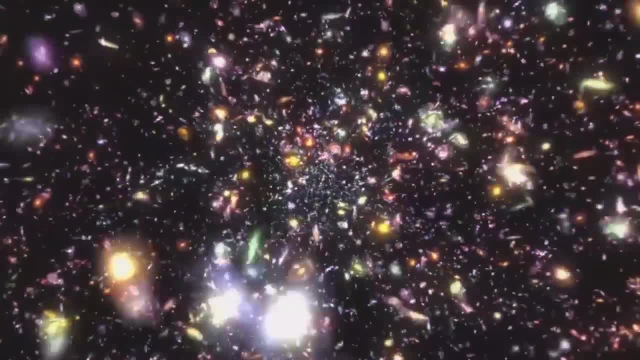 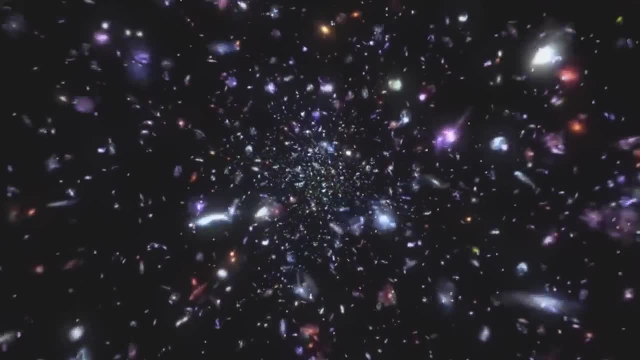 or, more specifically, the recombination era that occurred a few hundred thousand years into the lifetime of the universe producing light. as we know, it is the limitation that determines the radius of the universe, And so if we look at the universe as a whole, we can see that the 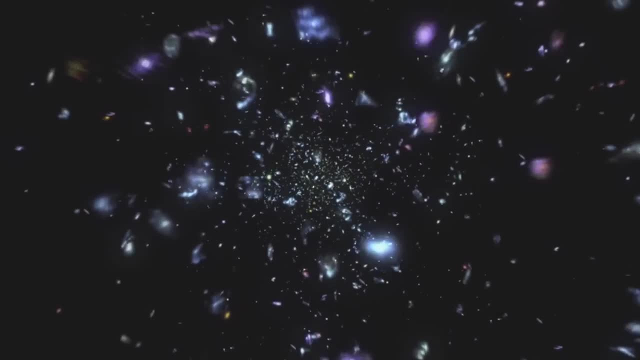 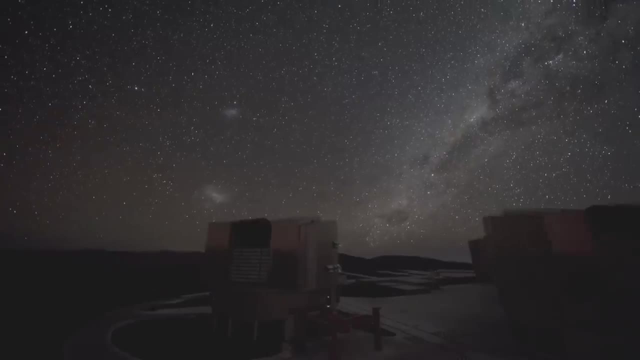 observable universe and therefore what we can see with telescopes, although we don't know precisely how big the universe is as a whole. But the fact remains that if we use powerful telescopes to look at objects that are many billions of light years away, which we have, 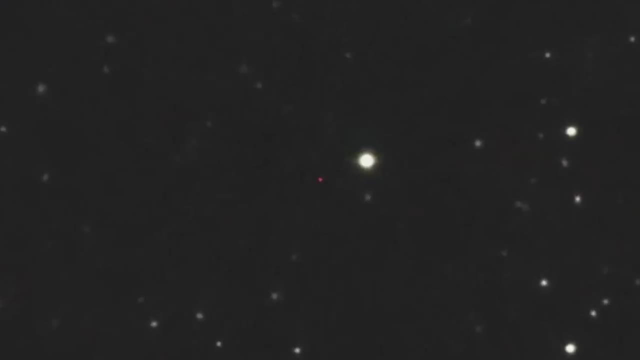 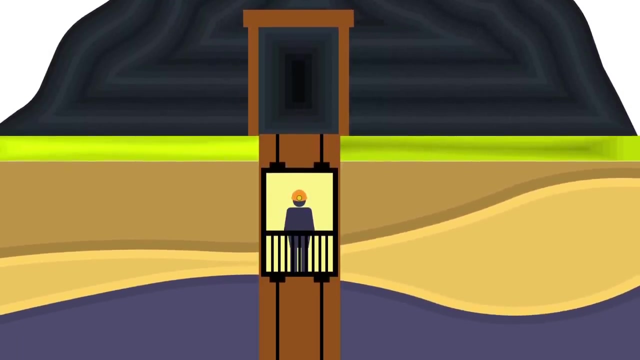 been able to do for a few decades. now we are looking at the first large-scale structures that developed in the early universe, and we get to look at them today. It's as though we could learn about the history of the earth simply by digging a deep hole in the ground and finding 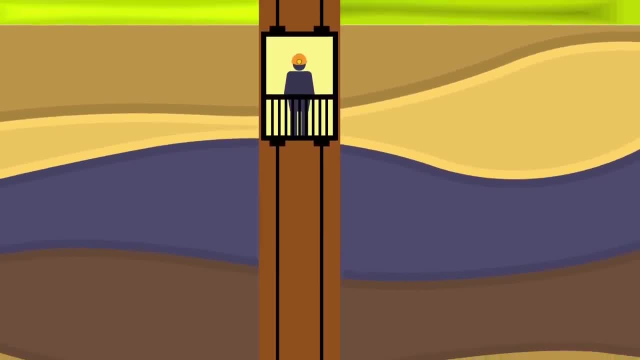 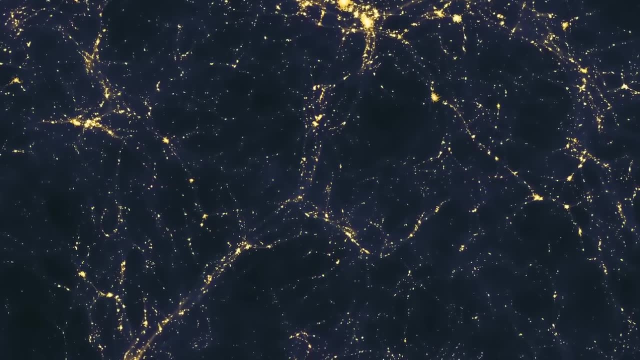 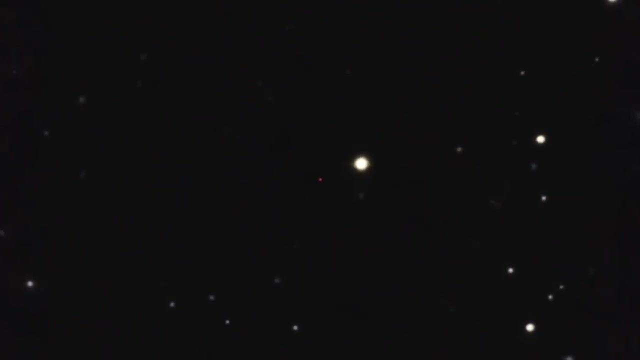 progressively older photographs of the earth as we go. This fortunate situation gives us the incredible opportunity to learn about galaxy formation in the early universe. When we peer this incredibly far out into the universe, we see objects called quasars, which is short for 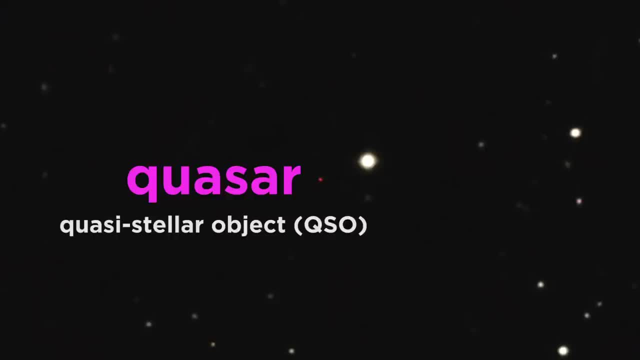 quasi-stellar objects, abbreviated as QSO. These were named as such because when they were first observed by early radio astronomy in the 1950s, we weren't quite sure what they were, since they appeared as faint star-like objects. 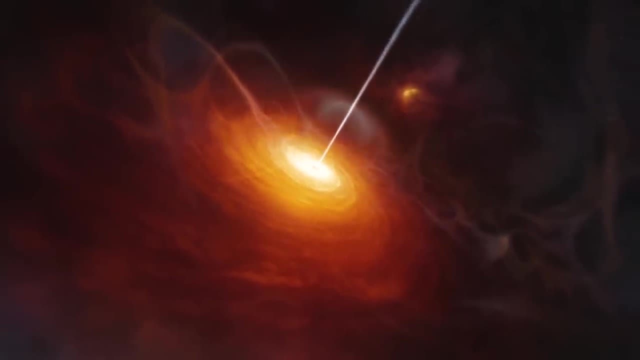 However, upon determining the extremely high redshift values for these objects, we began to realize that these are actually extremely luminous but very distant. active galactic nuclei, abbreviated as AGN. Essentially, quasars are supermassive black holes of millions or even billions of solar. 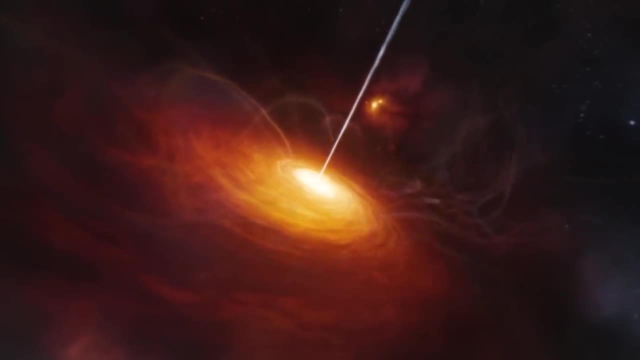 masses surrounded by an accretion disk of gas, often producing enormous jets of material that are ejected from near the surface of the black hole, perpendicular to the plane of rotation. This gas is racing around the black hole, which makes it very hot and bright. 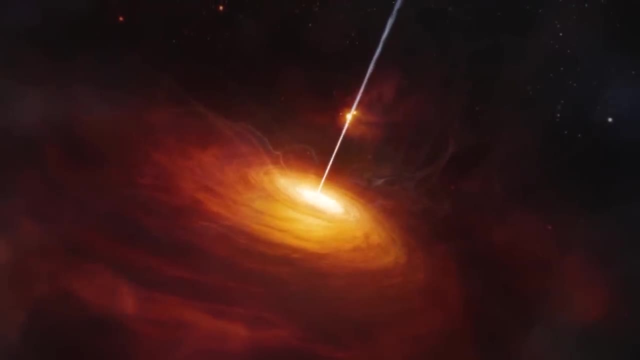 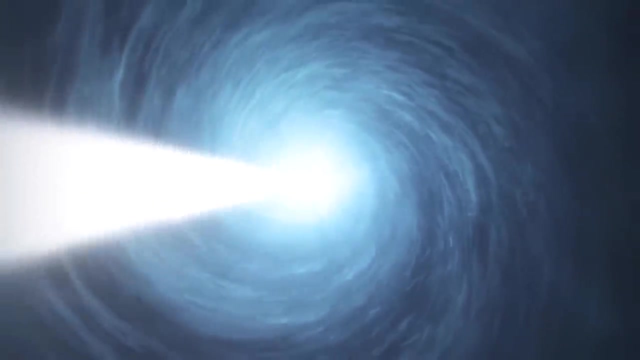 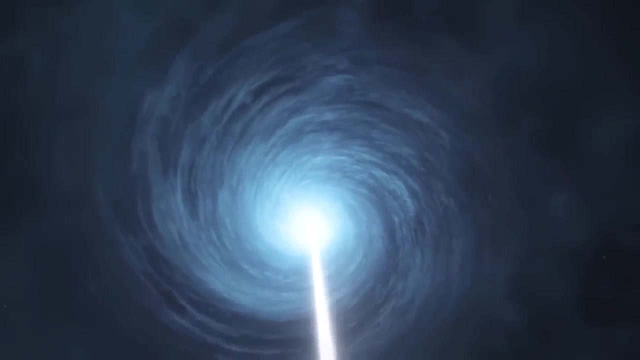 so bright, in fact, that a quasar is thousands of times more luminous than a galaxy like our Milky Way. That's what first made them so confusing, as, given their extreme distance, the apparent luminosity is closer to what would be expected for a much closer object. 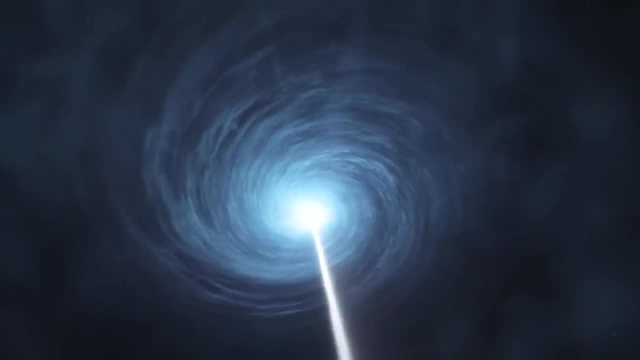 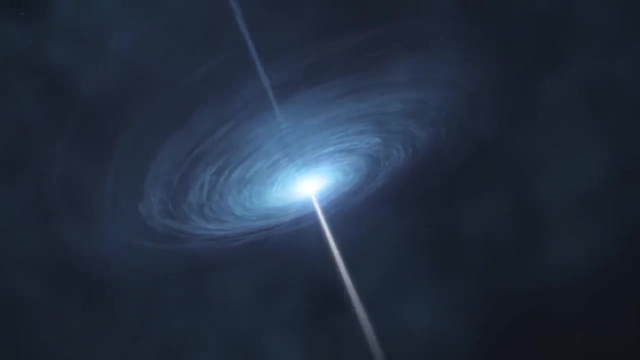 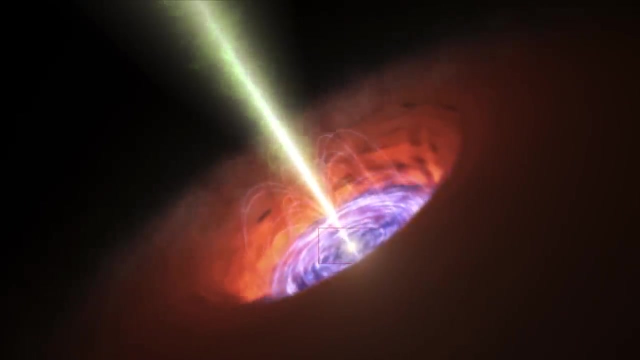 But now we understand that these are supermassive black holes that essentially serve as seeds for brand new galaxies to form, given the immense gravitational pull of the black hole. This makes sense in the context of galactic evolution, since there is a limited time after. 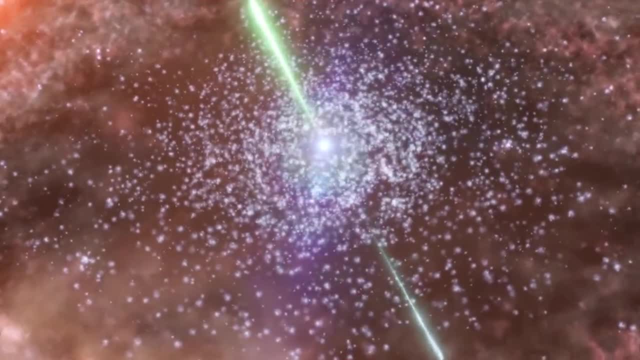 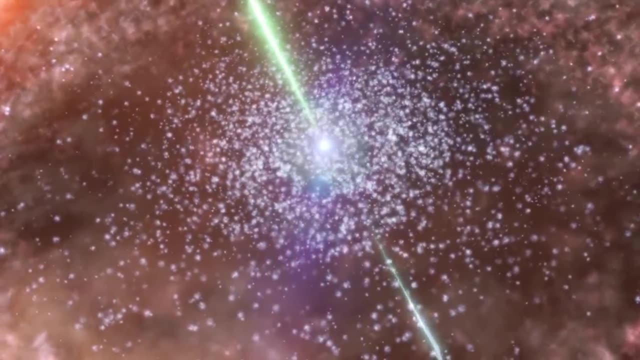 galaxy formation that an accretion disk can exist, as the gas near the black hole will eventually dissipate and the galaxy will become more ordinary. For this reason, most of the quasars we see must have formed in the early universe. on. 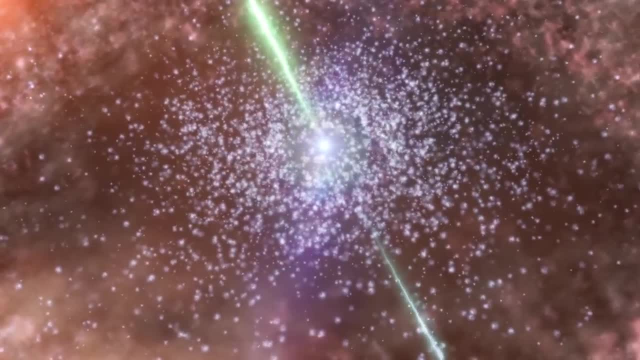 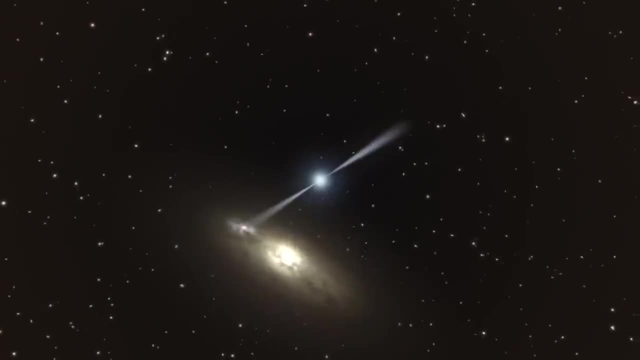 average about 10 billion years ago, most of which can be found within what is referred to as a host galaxy. To date, we have only found one quasar with no host galaxy, which is being studied to find additional information about the black hole. 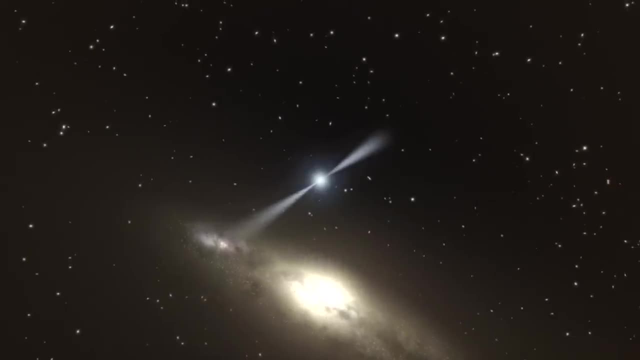 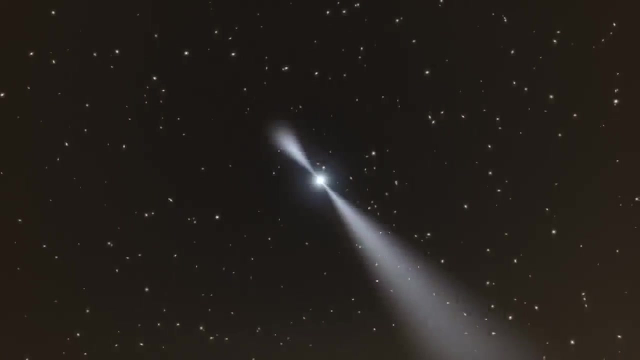 This is the first time we've found a quasar with no host galaxy, which is being studied to find additional information about the black hole. We've also discovered the mechanism of galaxy formation, such as the interesting proposal that quasar jets can stimulate galaxy formation, which will then merge with the quasar given. 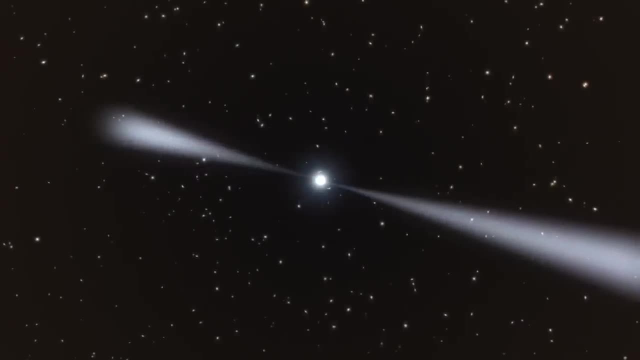 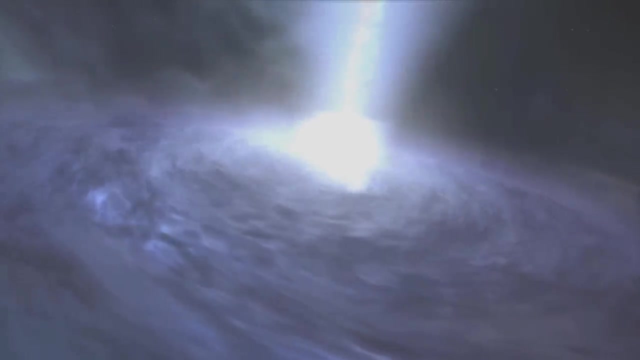 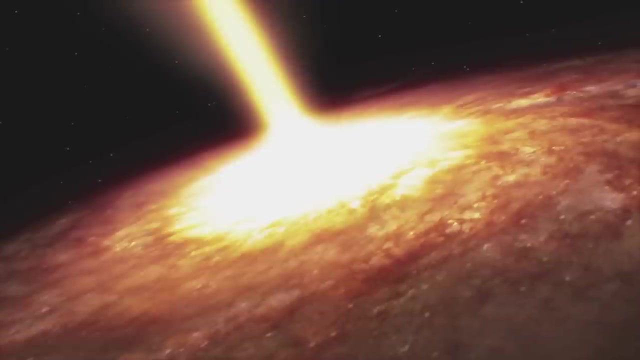 its supermassive status and the immense gravitational pull that results. But nevertheless, the very farthest quasars we have found represent some of the first large scale structures that ever formed, with the oldest forming when the universe was only 690 million years old. 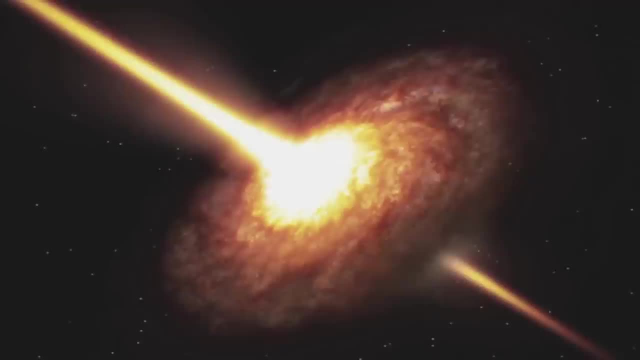 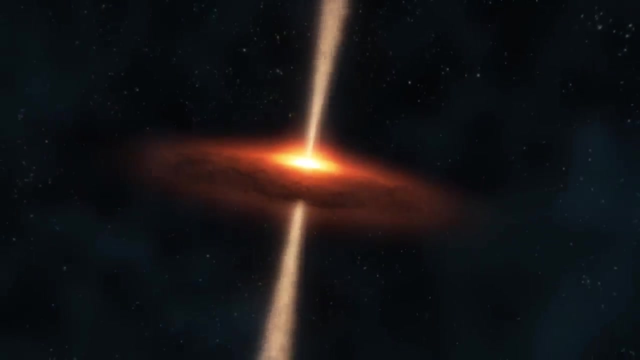 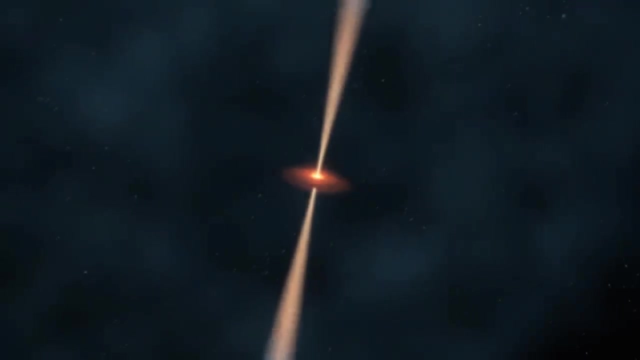 emerging from the so-called Dark Ages and its host galaxy must have been one of the first to ever form in the early universe. Such quasars from the very early universe are typically surrounded by a giant gas halo extending many thousands of light years, from the supermassive black hole consisting of 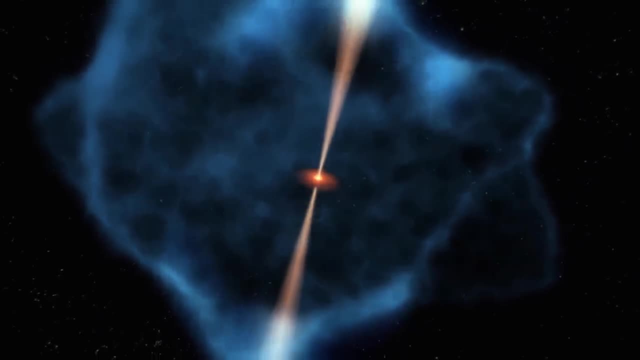 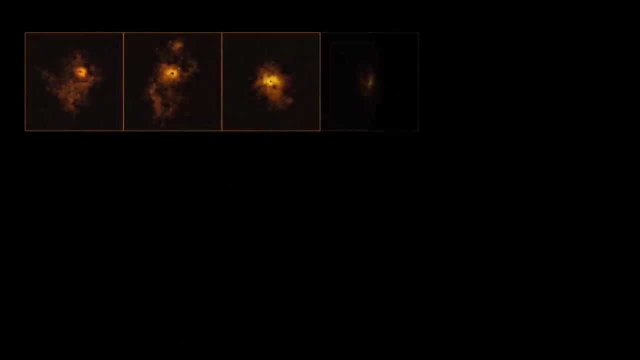 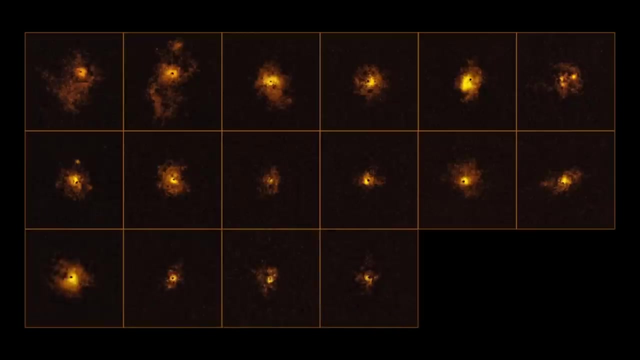 cool and dense, but glowing, hydrogen gas, shown here in blue. These halos sustain the growth of the black hole. Comprehensive studies of quasars have revealed such bright gaseous halos on a large proportion of the quasars, indicating that this is a common feature. 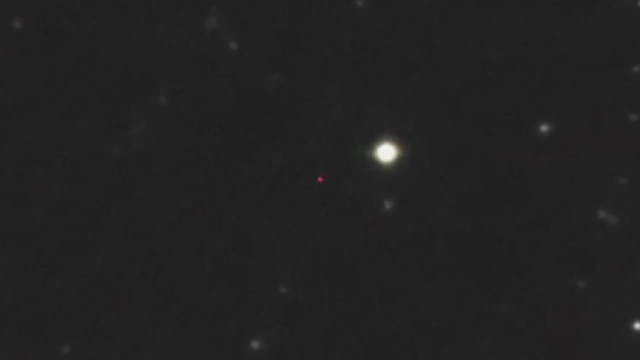 Once again. for a few decades after their discovery, there was some controversy as to what quasars were, but key evidence came by the way of X-ray astronomy, spectral analysis, and especially due to gravitational lensing, which we learned about in the previous tutorial. 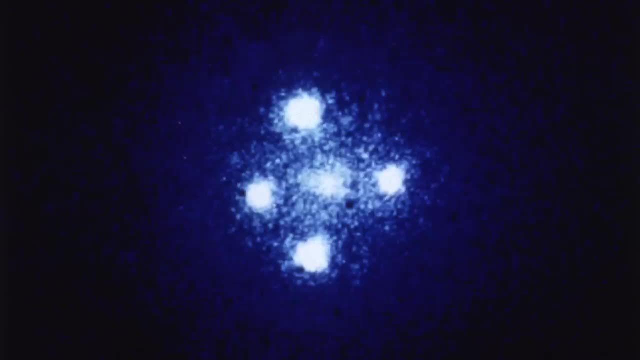 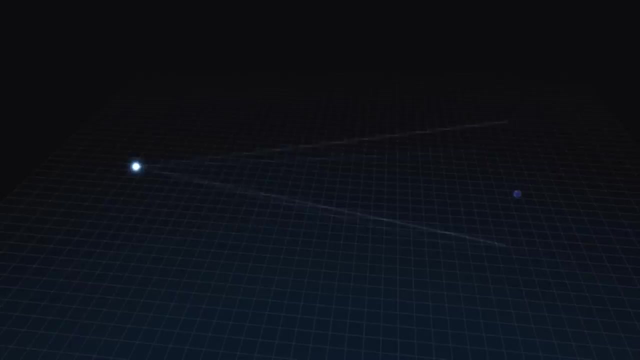 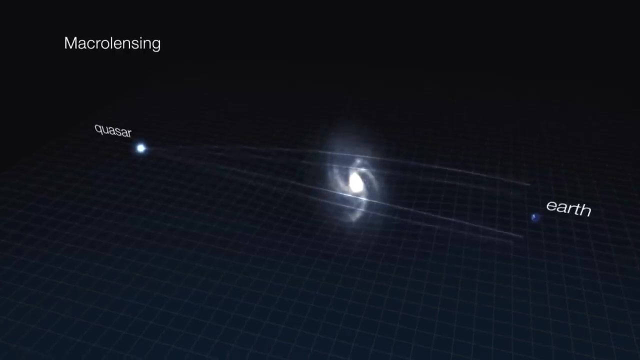 Sometimes the light from a quasar is bent around a foreground galaxy. In addition, more detailed analysis can arrive when we distinguish between macrolensing and microlensing. Macrolensing is the type of gravitational lensing we have been discussing, where the 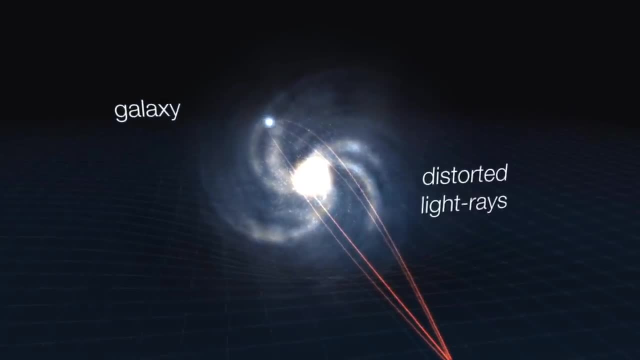 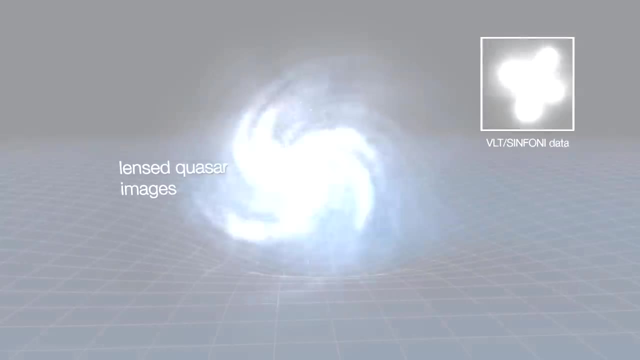 lensing object is very large, like a galaxy, which allows us to observe very distant objects. This is the phenomenon that would produce an Einstein cross, But individual stars are not the same. The stars within the foreground galaxy can produce additional magnification, which we 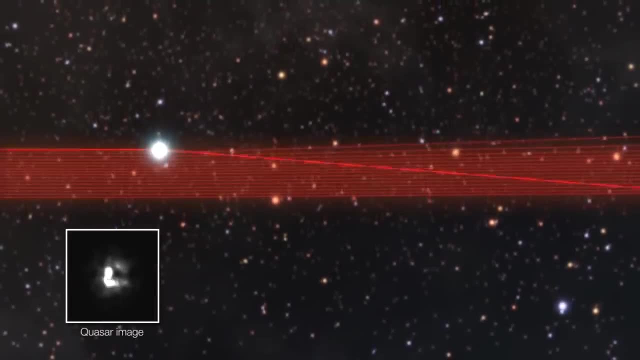 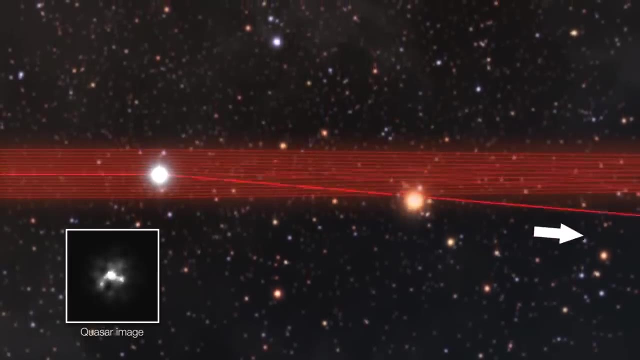 call microlensing, which operates by the same principles just on a smaller scale. As the stars move in the lensing galaxy, the microlensing magnification will change and this causes a flicker in the brightness of a quasar that can be measured and studied. 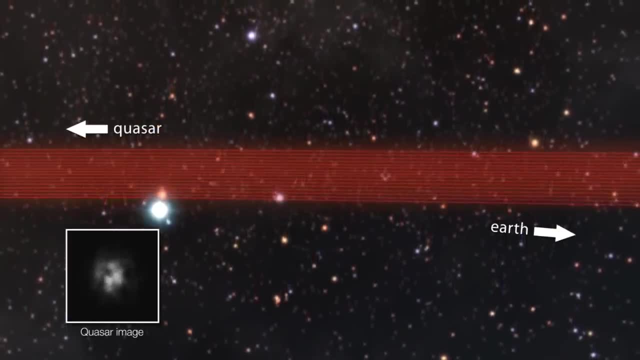 in order to gather additional information about the object. These days, we can employ an interesting strategy to study these distant objects. We can use the light from a quasar to measure the brightness of a quasar. We can use the light from a quasar to measure the brightness of a quasar.